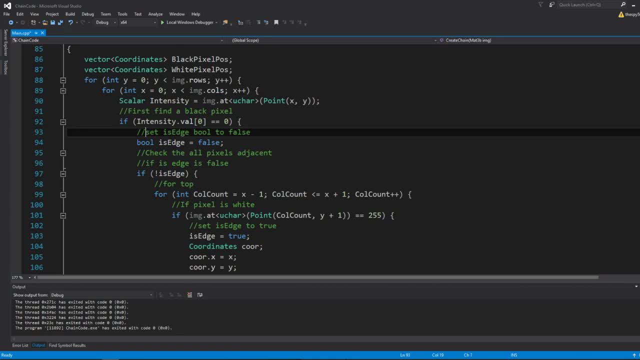 If the intensity equals zero, that means we find a black pixel. 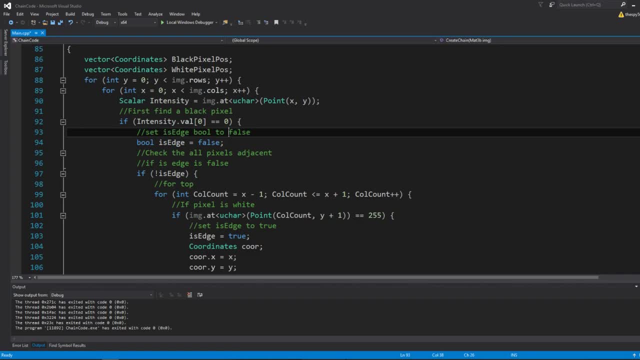 And then we have a boolean that's called is this pixel an edge, and we first set that to false because we don't know. 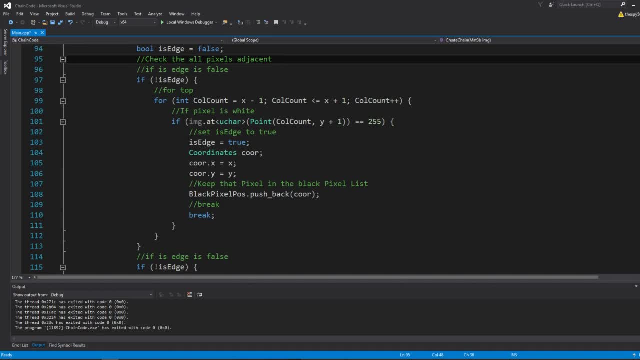 Then we check all adjacent pixels. If we find one white pixel, then we can assume that it is a pixel is an edge. So once we find that edge as equals true, we get the pixel, we get the coordinates of the pixels. 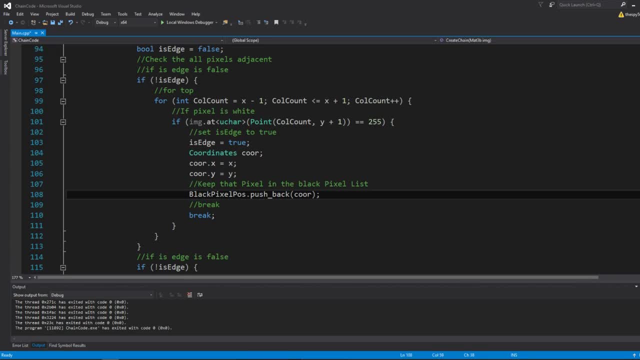 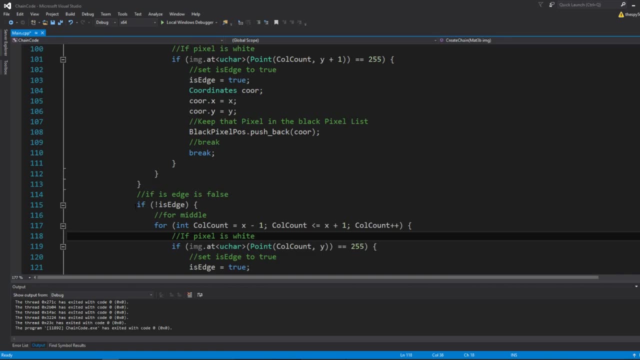 We're working with, and we push back those coordinates into our vector, and that coordinates is a simple data struct I created that just needs to flow. And then it'll skip the rest of the calls, checking the adjacent pixels because edge as is already equal to true. 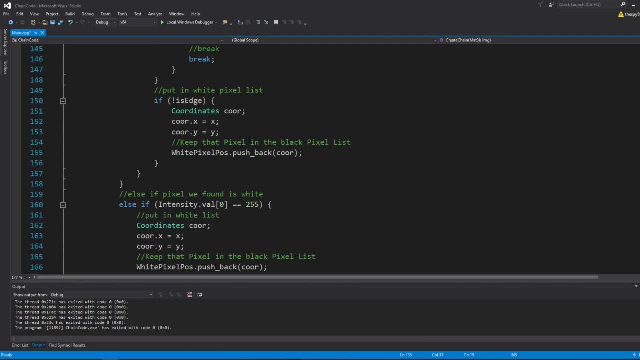 So it won't check the middle row, and it won't check the lower row adjacency for pixels. So in a picture, I can describe how it's checking it. 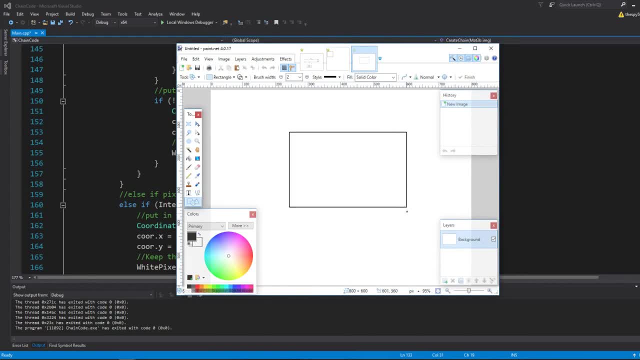 So if we find pixel, if we find that pixel, the first thing this program is going to do, check. Oops. 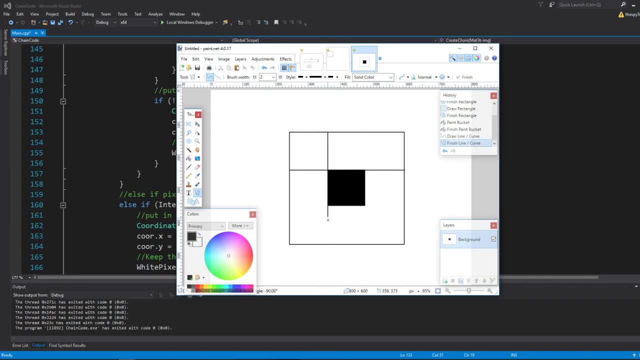 All right, that's good. First check. 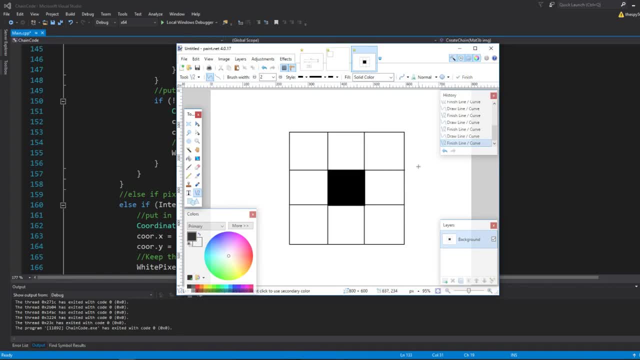 Top three rows, so we'll look here, here, here, oops, here, and it'll check here, check here, check here, and it's just looking for black pixels, here, here, and here last. So if any of those are white, then this pixel is considered an edge, and it stays. So it's like that. 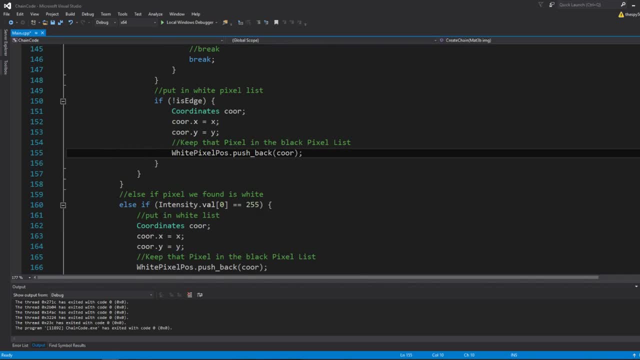 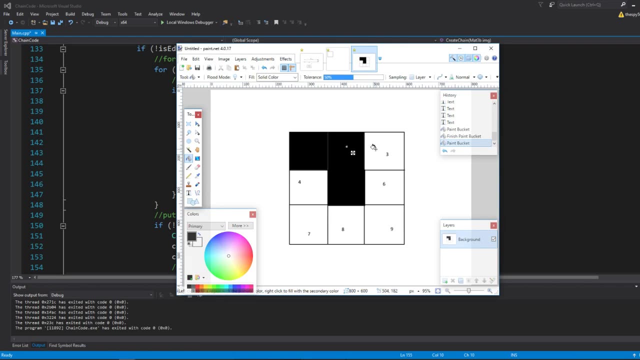 Now, if none of the pixels, if all the pixels are black, then we can say that this pixel is inside image, therefore it is not an edge. 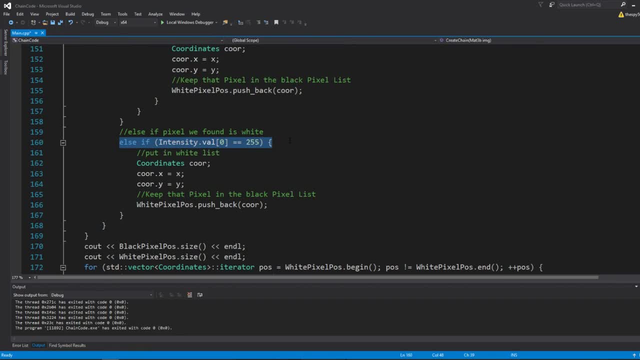 And then my last check is if the pixel we're checking, first of all, is white, then it's not an edge, it's just a background piece. So we get the coordinates. And then we push that into the white pixel vector. 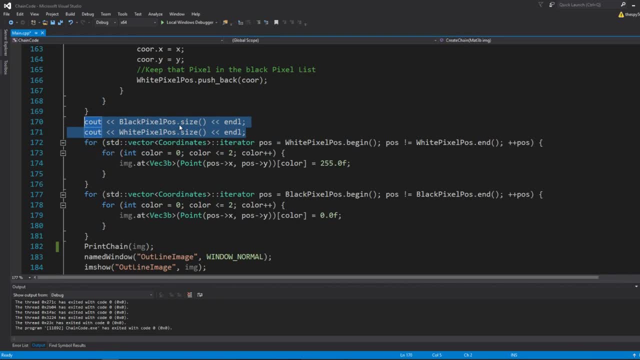 I print out the sizes just to see how many black pixels ratios we have to white pixels, because if there's more black pixels than white pixels, then my program wouldn't be working right. 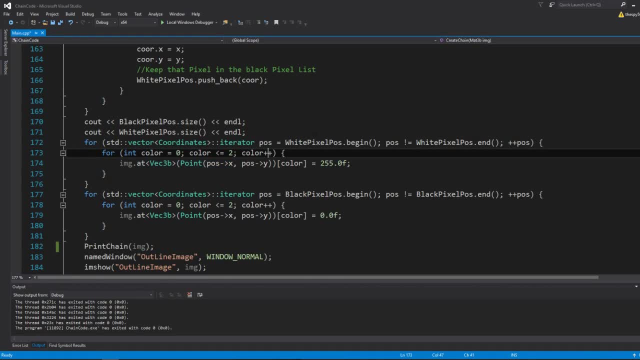 Then I say, okay, at those positions, we found all the white pixels that I want, or at those positions, we found all the white pixels, like the non-edge, I want you to fill them in with the color white. At all the . We're going to take the white pixels that were found to be edges, keep them and fill them in as black, just in case anything happens. 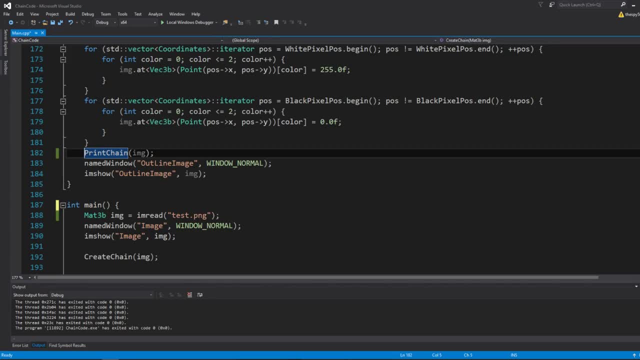 Then I move that to get the chaincode, and after the chaincode happens, or after we get the numbers for the chaincode, I print out the image. We're going to go up to the chaincode. There's the structure, the float X float Y. All right, so the first thing we have to do is find the first pixel. 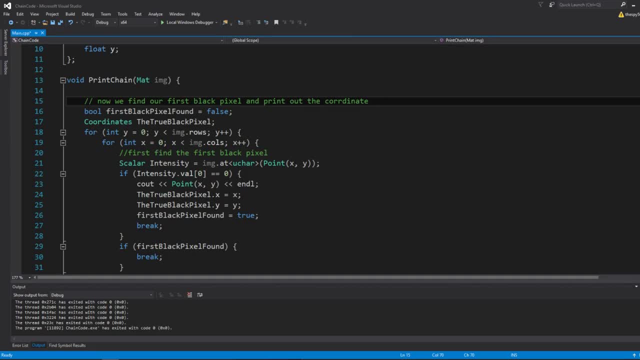 We had to find the very first black pixel to start. looking into our image because we're assuming that the image is a complete shape with no gaps 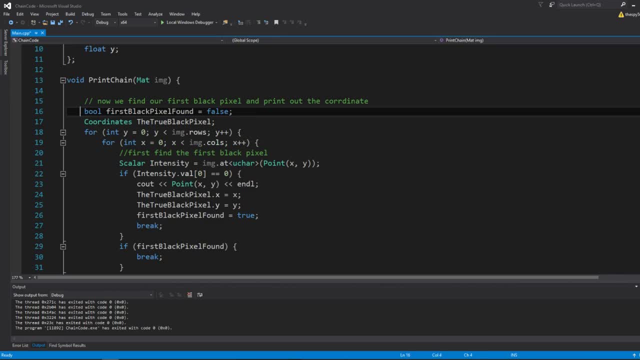 so we haven't found the first pixel yet just in case the user puts in a blank pixel none of this will run get the coordinates for that 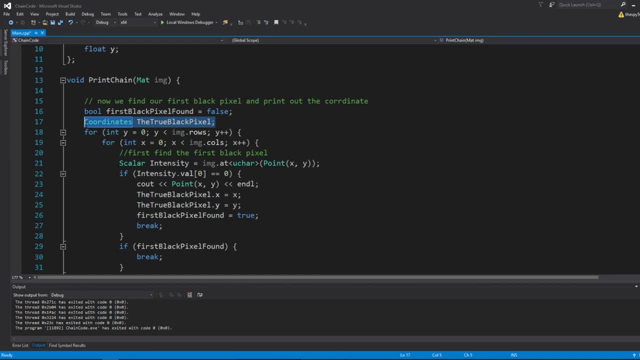 or we create a coordinate variable to hold our x and y for that black pixel then we get the rows and columns so we iterate 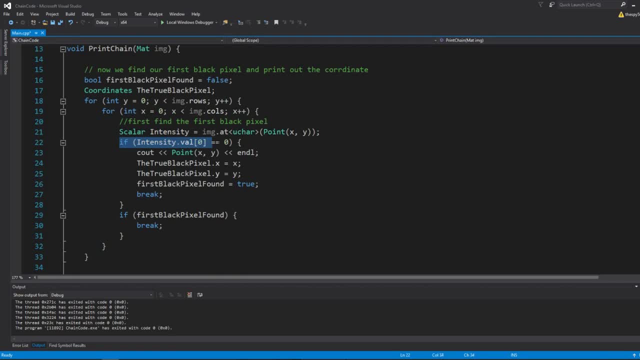 through the entire image we look at the intensity of every single point in our new image and then we try to see okay if we found that the intensity at the value that we're looking at is 0 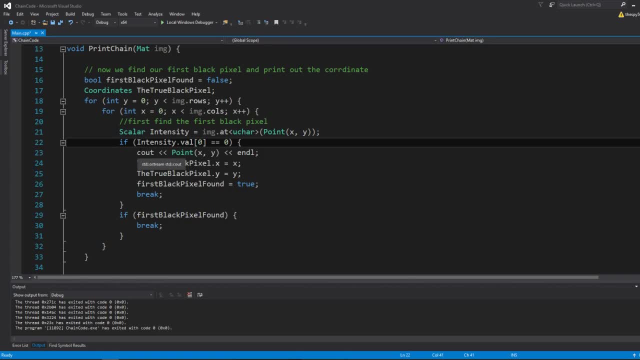 then that is the black pixel we would start this 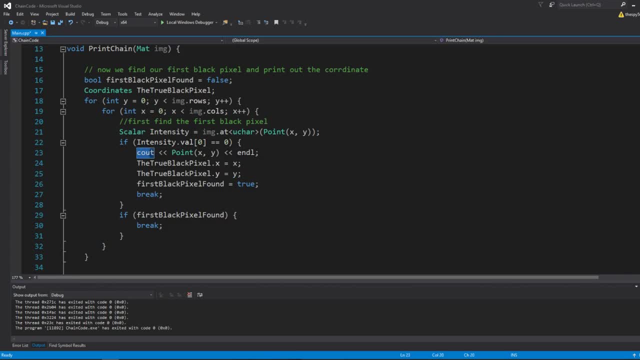 this test from so we print 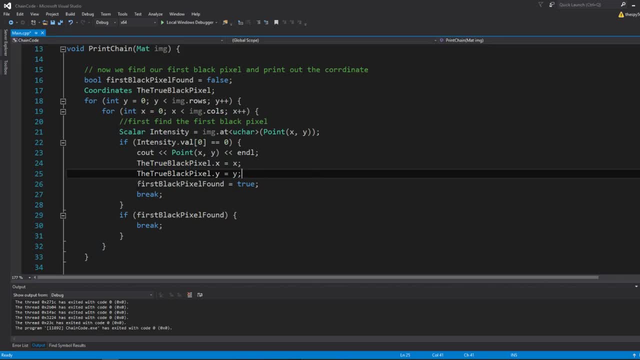 out the point we get the pixels x and y and then we say it's true, break out of this loop 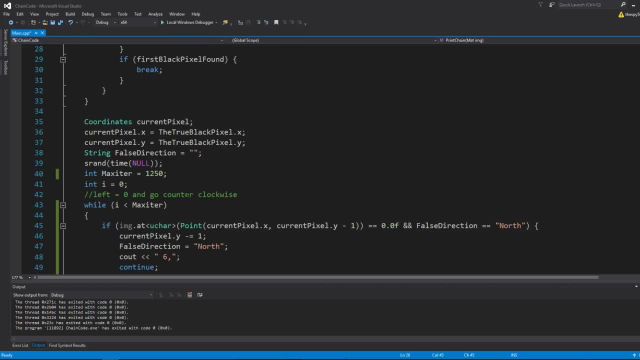 if we found it, break out of the next loop so we can get out our 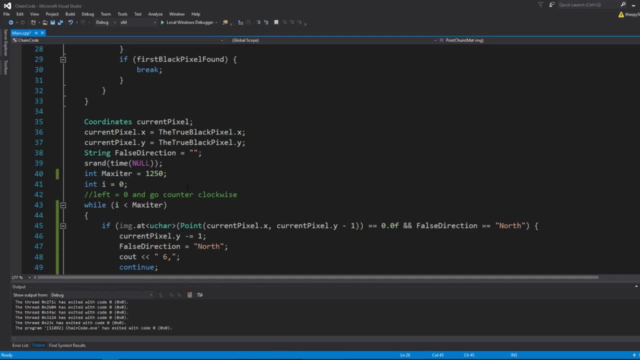 embedded loop yeah I think it's embedded loop is what it's called 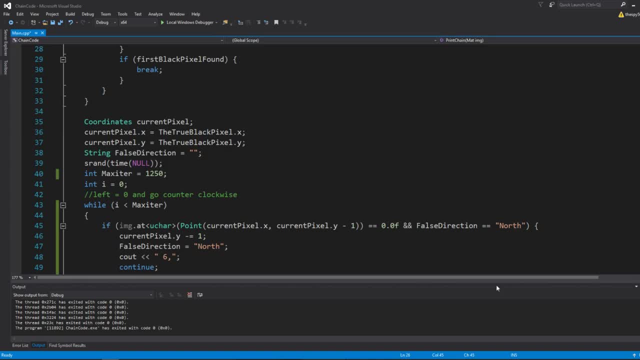 then we go on to getting our train code so current pixel we get some coordinates and then we just say our current pixel equals our first black pixel 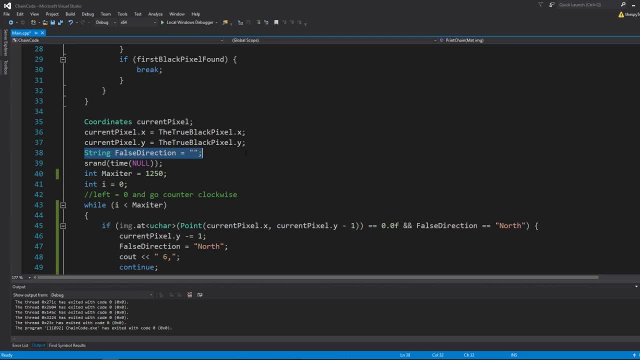 we found is x and that's y 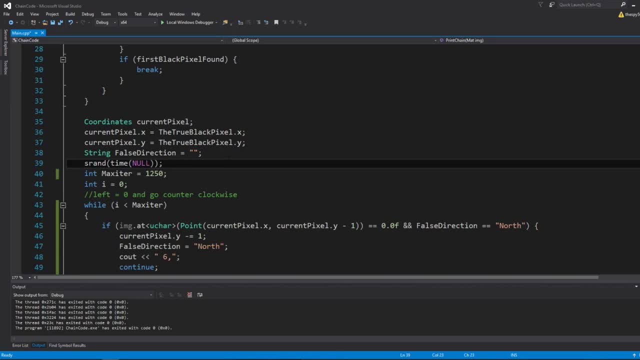 we have a string called false direction which we'll see you'll use later random time which I forgot to give max iteration max iteration max iteration 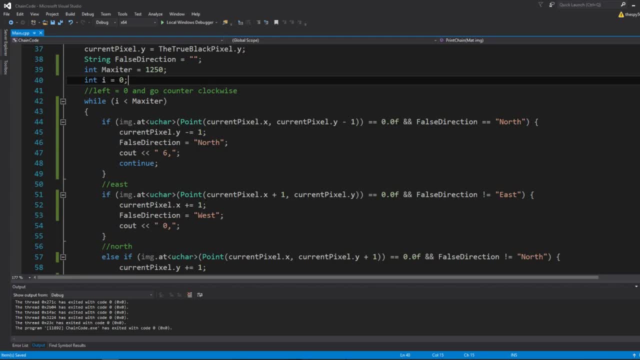 just in case it gets stuck into a loop and in the so while I list the max iteration it's set at a pretty high number just in case 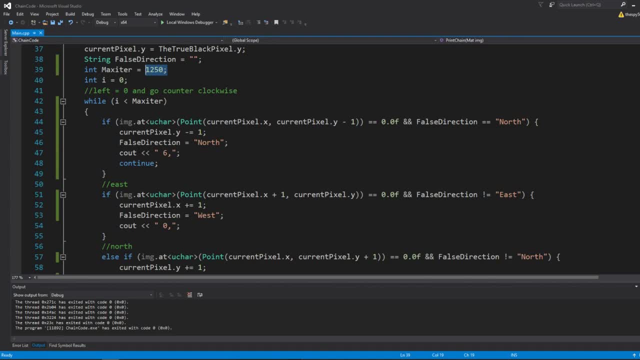 it goes overboard and you can get rid of this whatever and just put true what I found with some images it could go into a loop, so I made this a max iteration so it stops 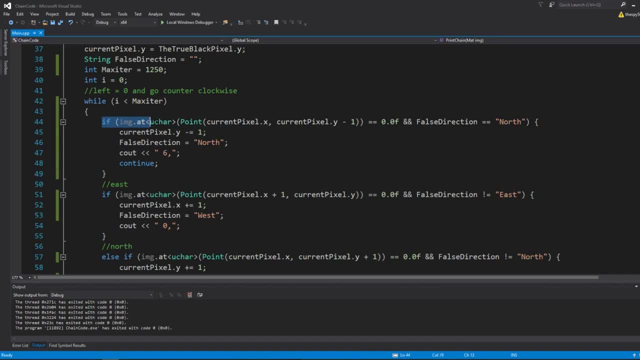 so if at charpoint if at the point we're looking at right so Back to this image. 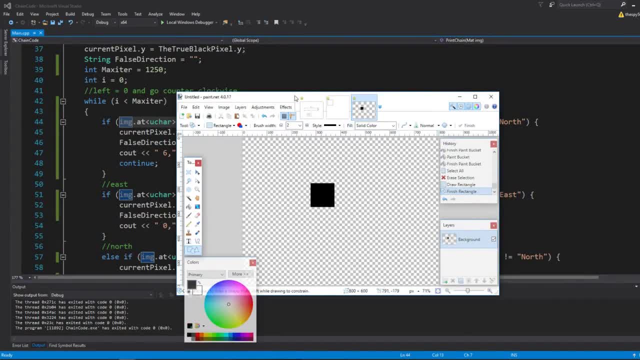 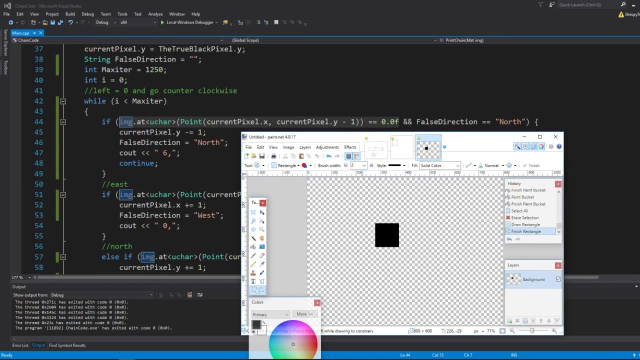 Okay, so if we're looking at this pixel, right, this is saying If the pixel we're looking at below is 0 and the false direction is north, then move the pixel south. 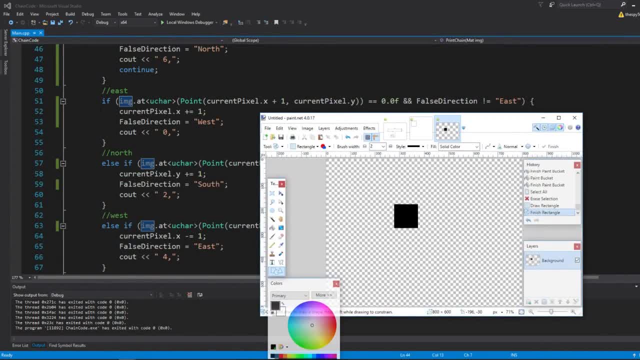 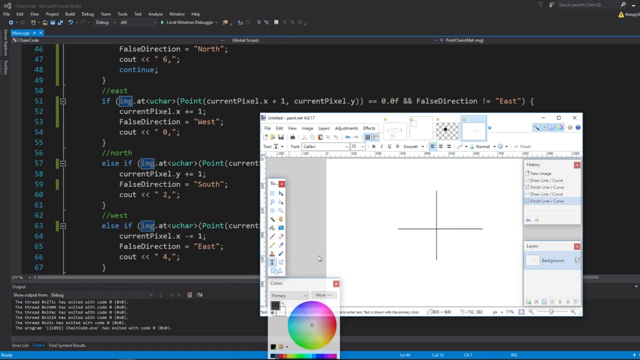 But that's a condition for later. So let's actually start at this one. This is where the actual check will start. If we remember, from earlier, I'm going to be using a absolute coordinate direction of the four basic cardinal rules. East will be 0, north will be 2, west will be 4, south will be 6, and you always want to check it in a counterclockwise way. 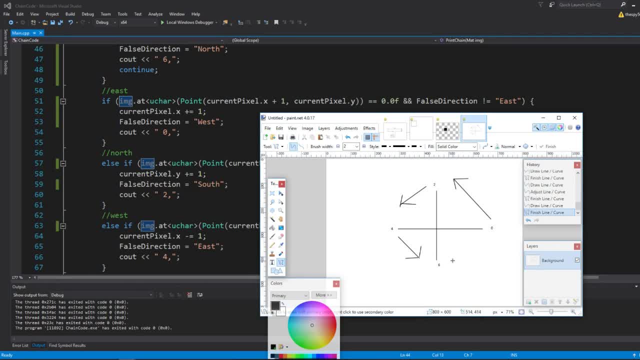 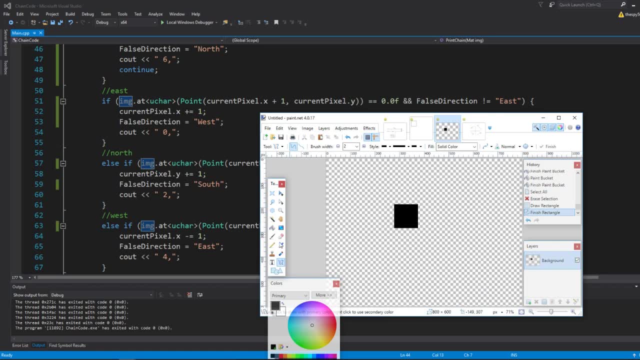 What this means so at the very beginning of our picture, this is the current pixel that we're at. 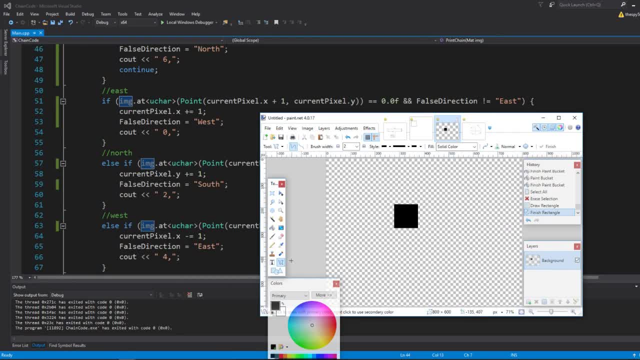 And I'll say, okay, I'm going to first look east of this pixel. Is that pixel a black pixel? Is my current direction... is my false direction east? 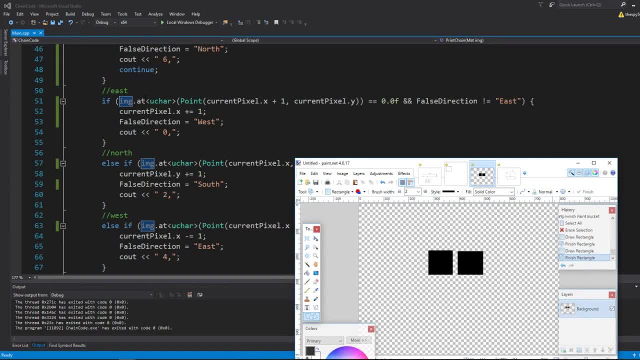 Which I'll explain later why we have that. So So, very first statement, it says, alright, let's look east based on these cardinal directions. Did we find a pixel with an intensity of 0? We found a pixel with intensity 0. 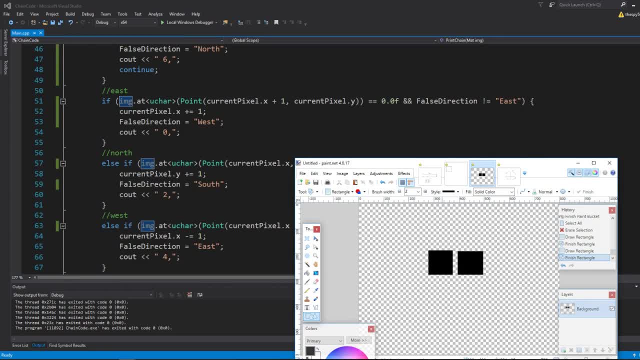 And the false direction is not equal to east because right now it's empty. So it says, okay, take the current pixels x and add plus 1 to it and make the false direction west. 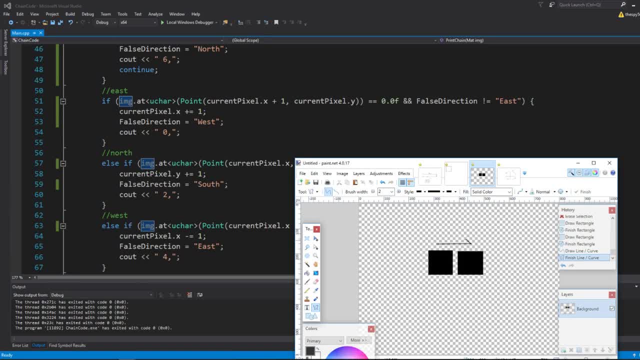 And what this is saying is we take our current points that we're looking at. We say, okay, now this is our current pixel, right? And we say that the false direction is west because if we don't say that, then the next time this pixel looks for its friend, say if we reach a corner like this. 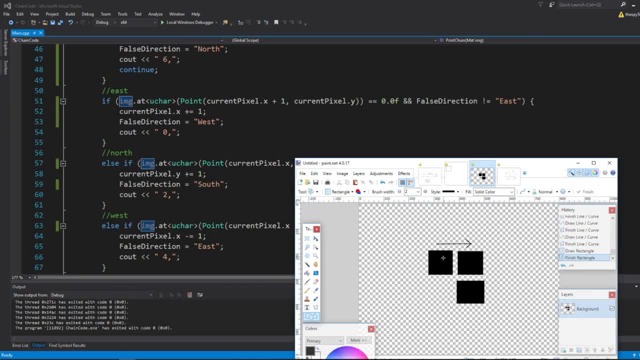 And we say, okay, we found east and we're like, okay, it didn't find east, west, and it goes back here. Back to this pixel and then it looks again east and then from here it looks west, east, west, and you get stuck in a loop between these two pixels once you reach a corner. 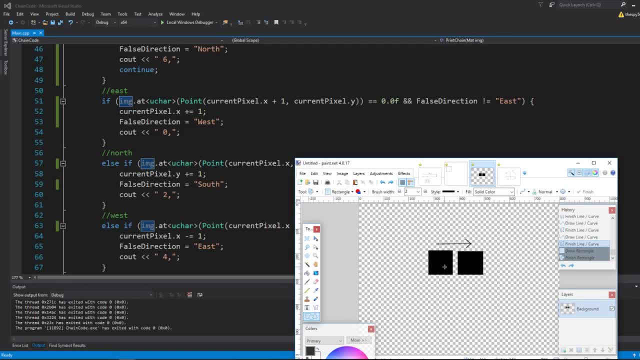 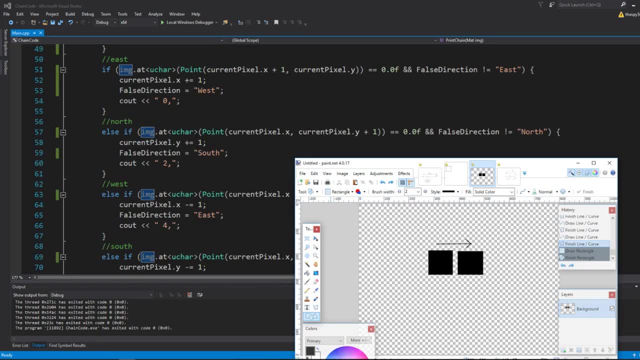 So we say the false direction is west, so it won't look back there, therefore it doesn't go backwards in how it tries to find pixels within the chart. So it's pretty much the same idea for the rest of them. 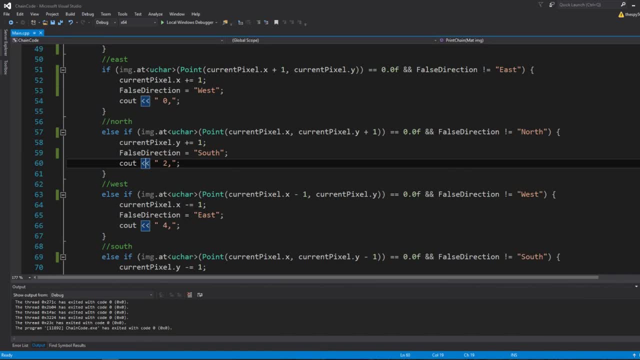 If the pixel above is black, then we go up. Or if the pixel... 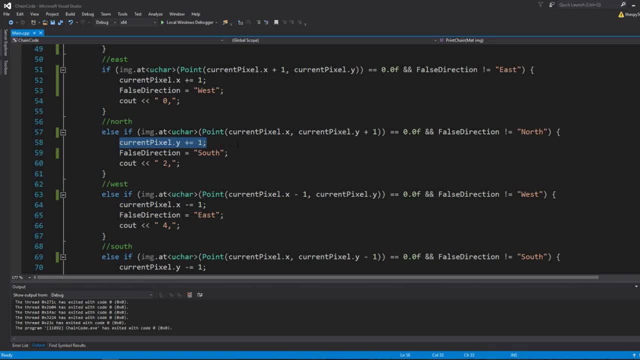 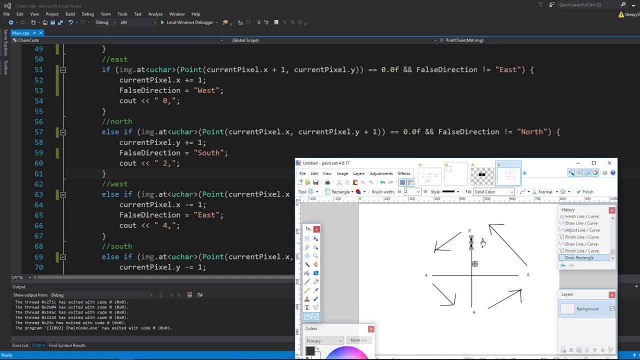 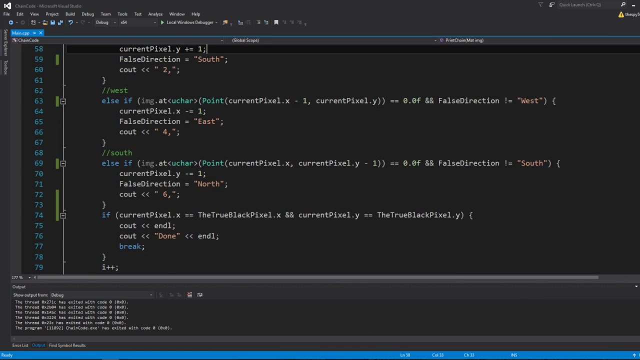 If the pixel above is black and our false direction isn't equal to north, then we move the current pixel north, false direction south, see out to, which is this again, see out that absolute coordinate. West, if the pixel west to us has a scale of, or an intensity of zero and the false direction isn't west, shift our current pixel to west, false direction is east, print out a four. And then lastly south, if the pixel below has an intensity of zero and the false direction isn't south, then the false direction is north and we move our pixel down one and see out six. 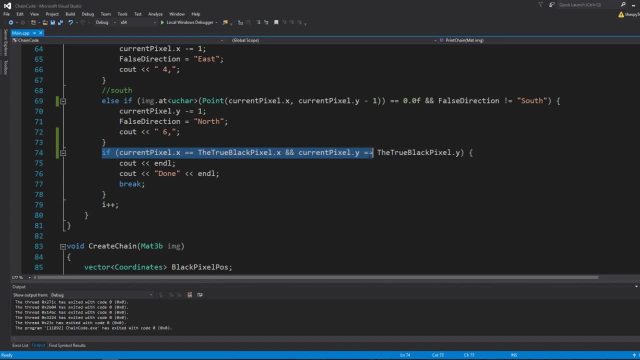 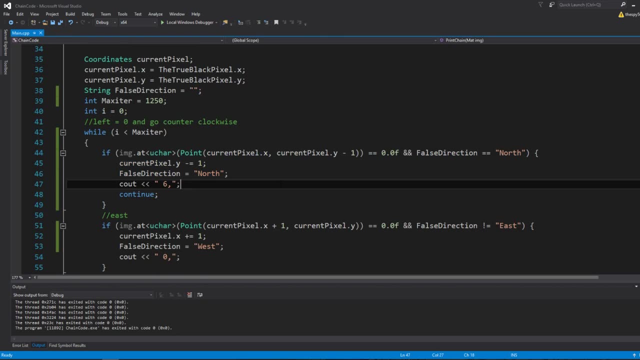 And then at the very end, if our current pixel equals our original coordinates, then we're done looking. And then we iterate one up. Now the reason I have this up here, and this is basically south. But check for south. 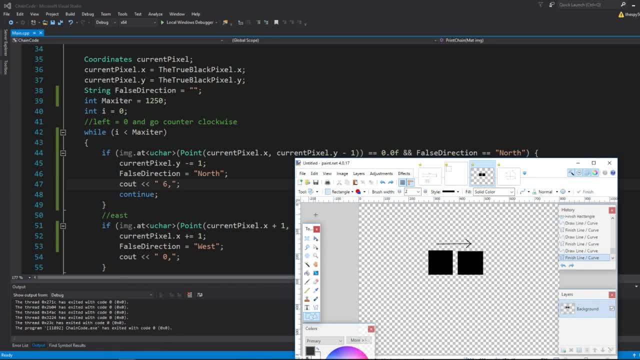 South, again, is if when you decompose, or if you, when you make the outline of the picture, you have a structure like this. 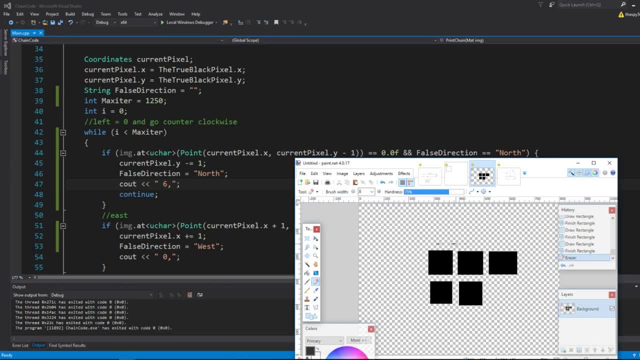 Pixels left. That. You can run into some problems. Let's assume we're at a corner, right? We decompose. Our square. But on one of the corners, we have a structure like this. So. These are white. 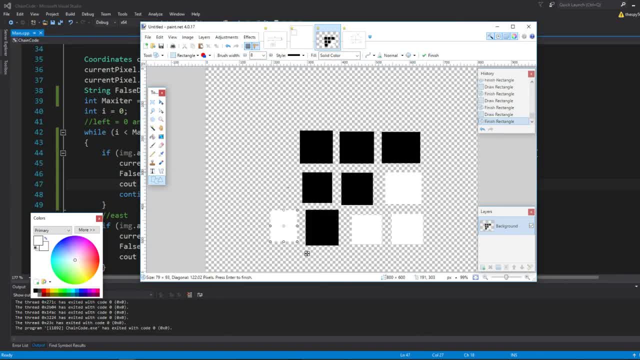 So when we found the image, we found that these are white. Everything on the outside is white. 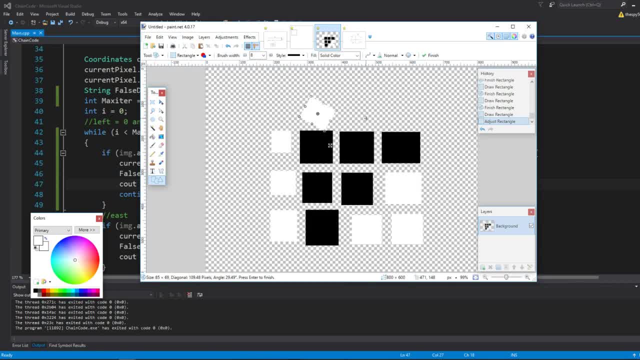 but this pixel right here was found to be an edge 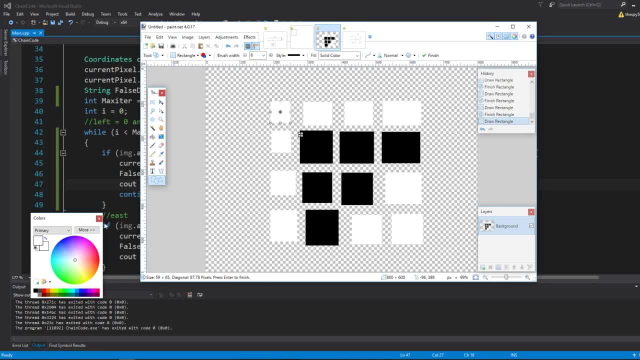 and that's something you need to add in more cases for to fix but in case you can't 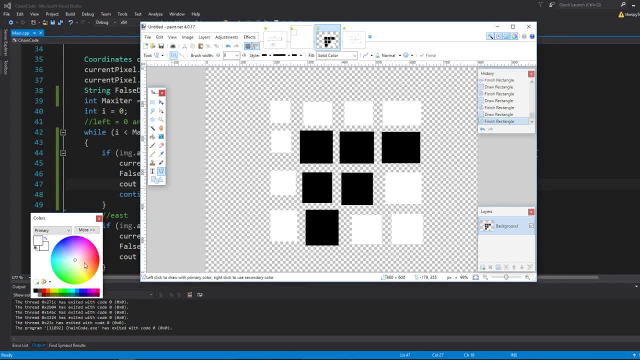 what happens with this error is it'll start from it'll start from this pixel and go to there 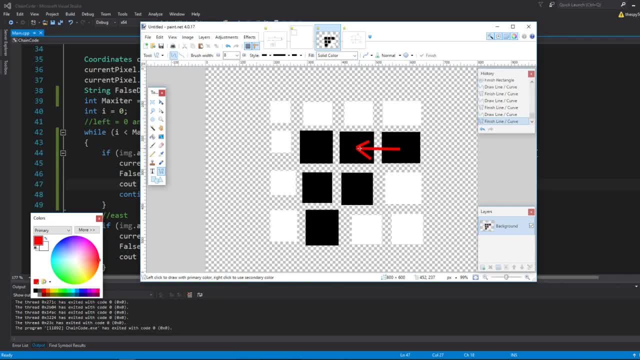 and then this pixel will look and say okay my false direction is east so I can't check that pixel this one's white this one's black so I'm going to move here 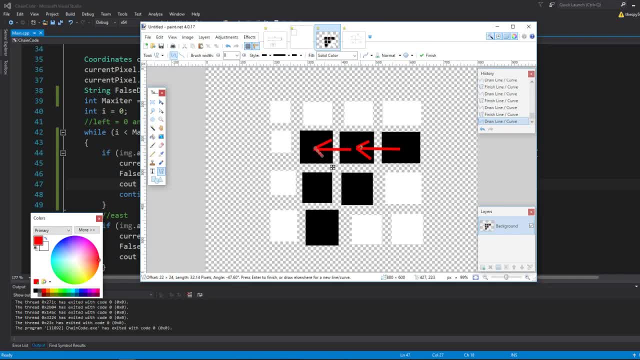 it moves here my false direction is east so I ignore this pixel 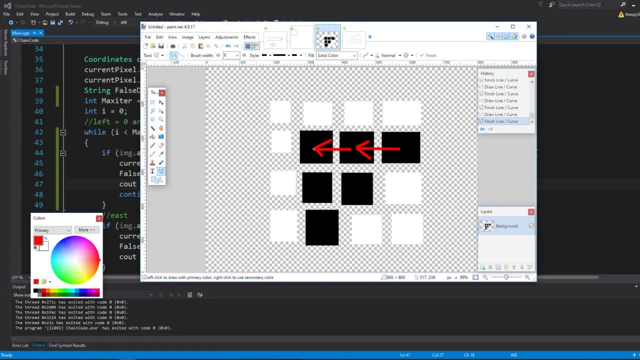 that's false that's false that's false oh I can go south now 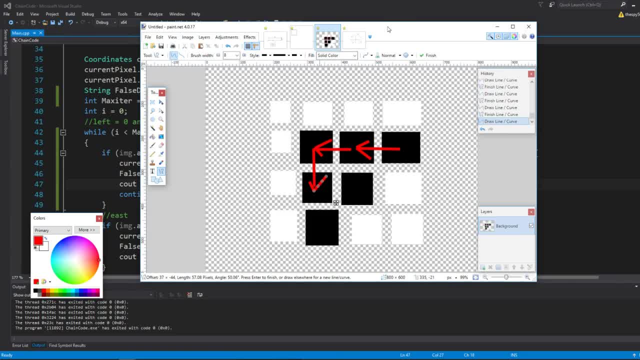 now if you didn't have that condition I have it above 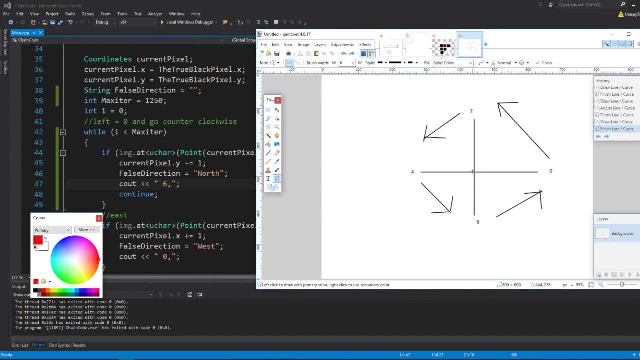 what it would say then is every time we look at a pixel it always checks east, north, west south, east, north, west, south it always starts at east 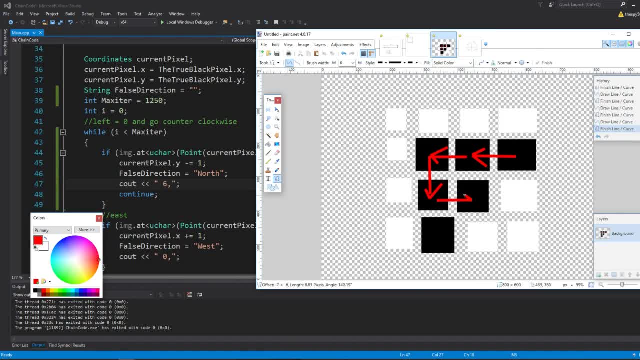 but if you do that then it says oh this is a pixel I'm going to go here 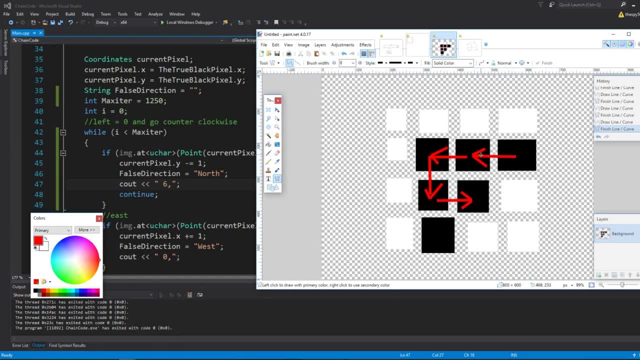 and now my false direction is west it's like okay I got white here and then it was like okay I have north it goes there now my false direction is south now I go east now my false direction is west and then you get stuck in this endless loop right here 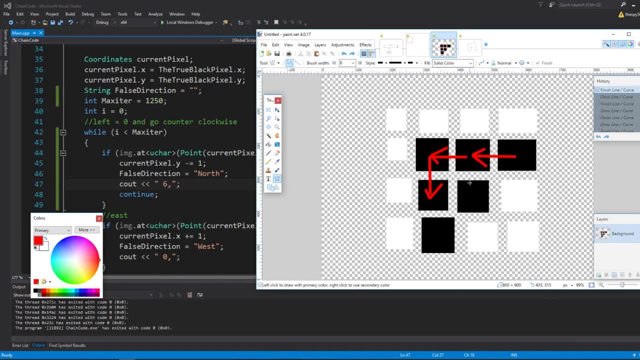 so what you do instead to bypass that problem is since south is always going to be the last one it checked 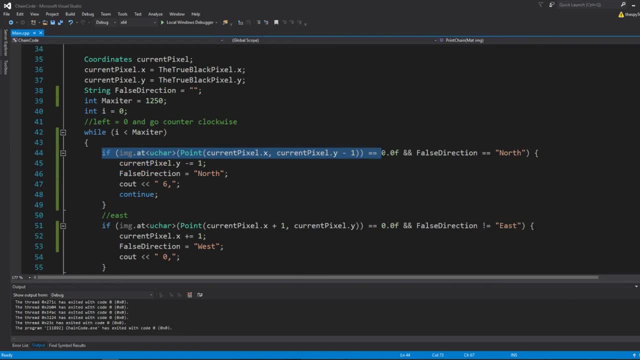 what this is saying up here is that if south was the last thing checked 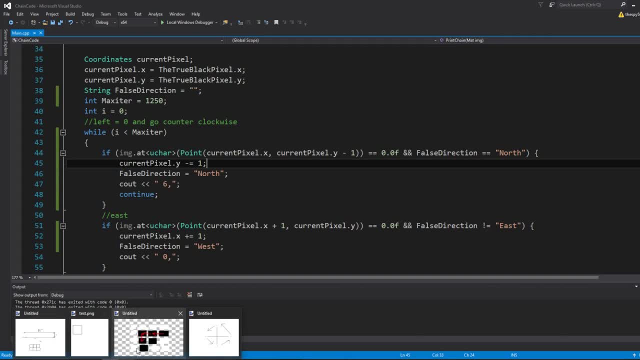 we're going to start checking at south first before east which in picture terms is we start checking here oops 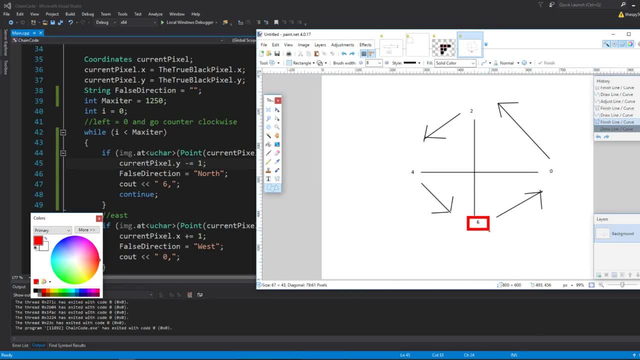 change that to a square we start checking at this one and then move counterclockwise and with and because we do that it'll say oh hey look here's a black pixel and then we're going to check at south and it'll start going down as intended and ignore this pixel so that's how the code works and then at the end it doesn't return anything 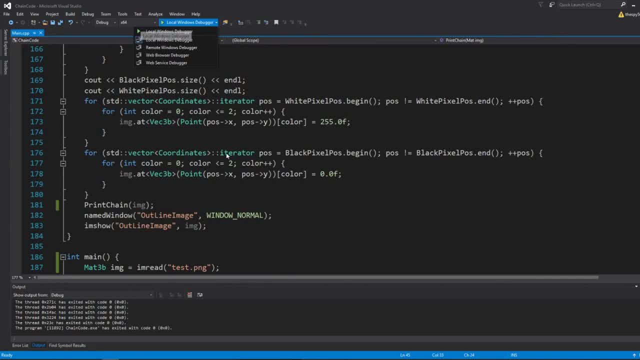 um it just it just prints out 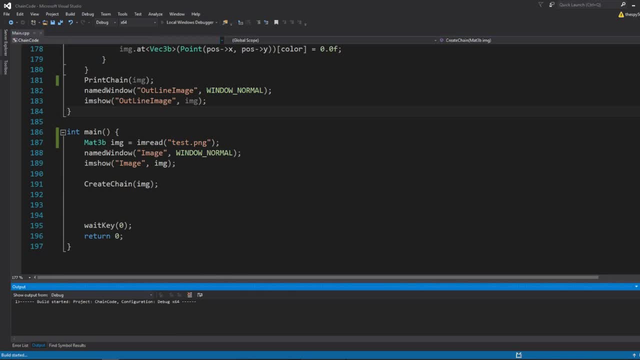 I'm going to first start start this with the test image so it decomposed the image and this is what it came out with and OpenCV has this weird thing where it says openCV has this weird thing where it says openCV has this weird thing where it says openCV has this weird thing 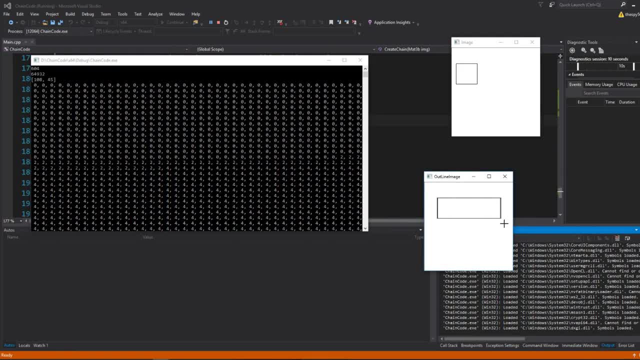 with um or at least not OpenCV 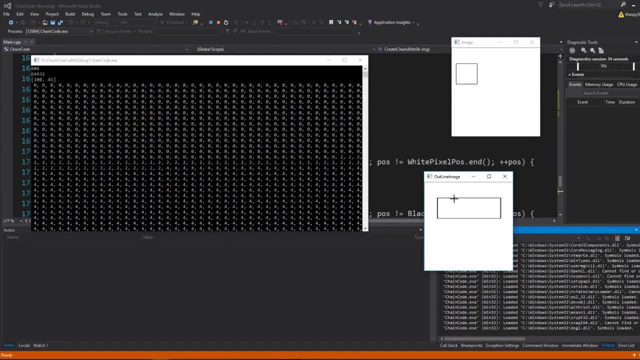 sorry my code the deconf sorry the outline code I made 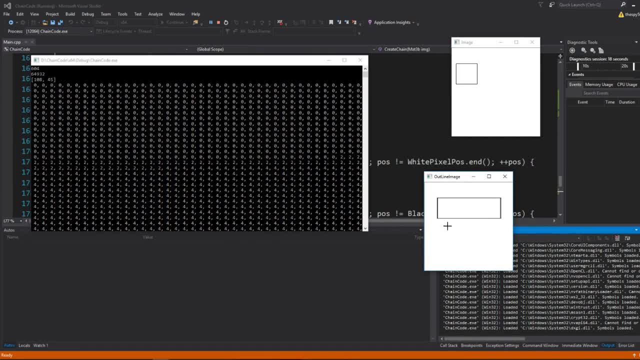 is doing this thing where it makes it bigger but basically what it's saying is okay we're starting at this pixel all the way down here 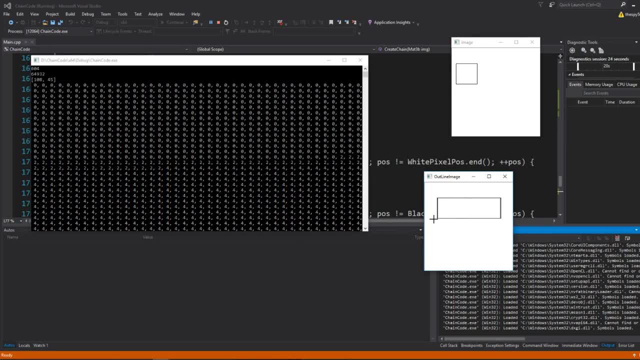 right we're going to move east 580 times 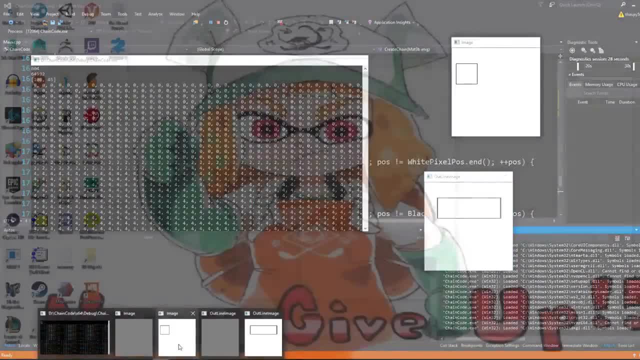 so then it's back here 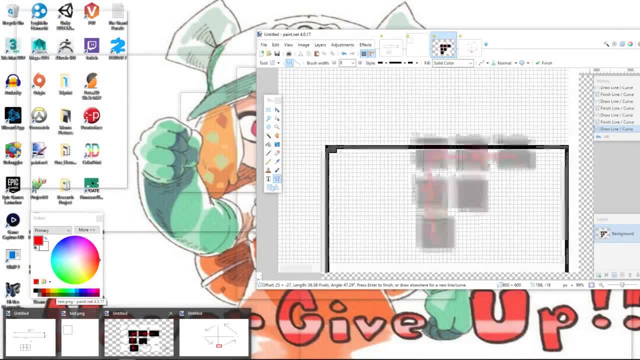 let me see if I can draw it bigger um 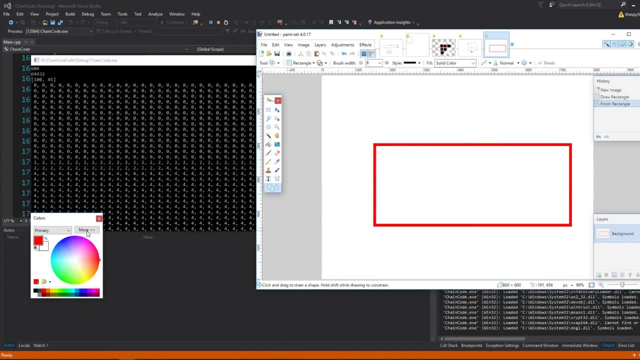 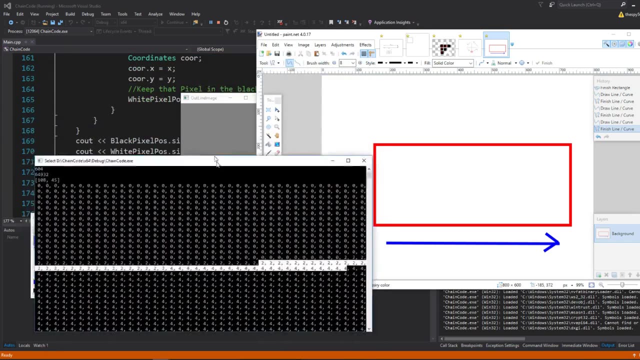 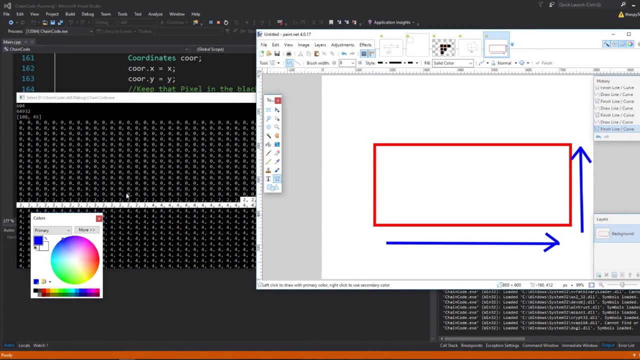 so it's saying I'm going to move east 500 times and then we see that shifts two right here two two two two two two is north so it's going to shift to 50 or 60 something times see here at four then it goes east then it goes east the same amount of time sorry west the same amount of times 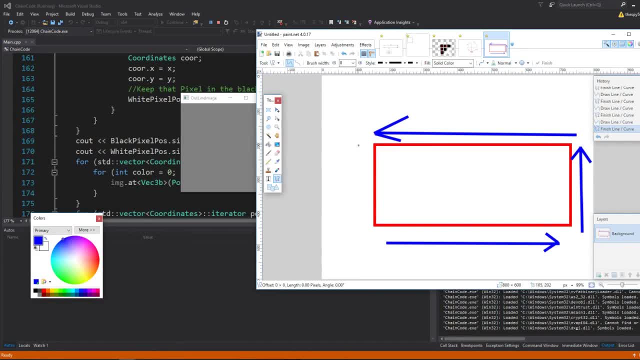 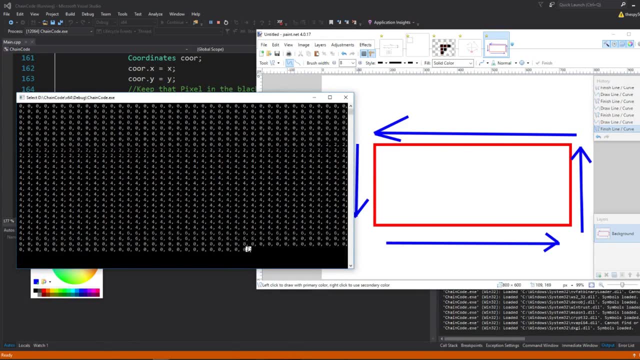 and then we have the sixes here shift once our max and then it keeps going in a loop and then it hits the max iteration then we're done so 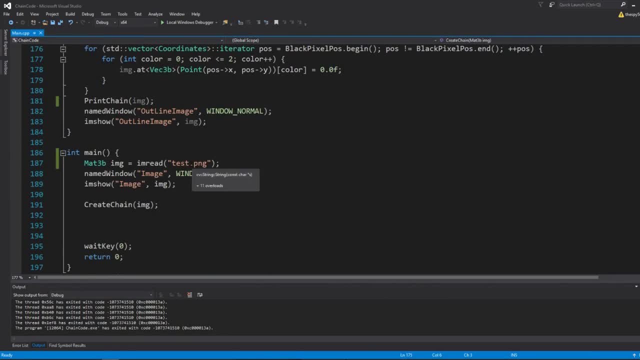 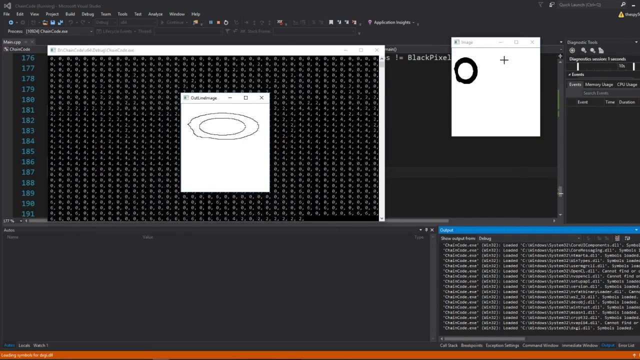 now let's test it on something that's oops the other image I have saved all right so this is the image that we start off with this is weird looking donut ring 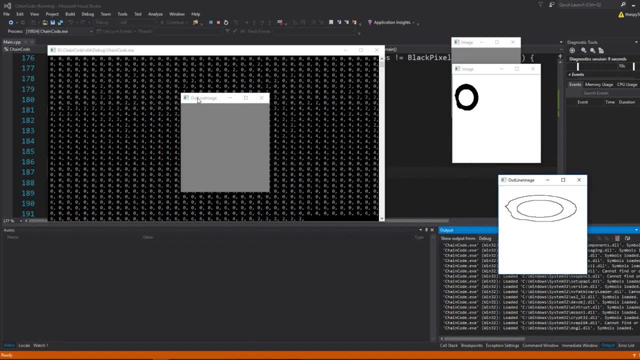 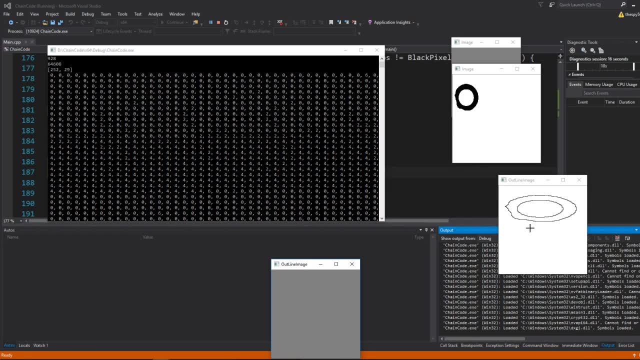 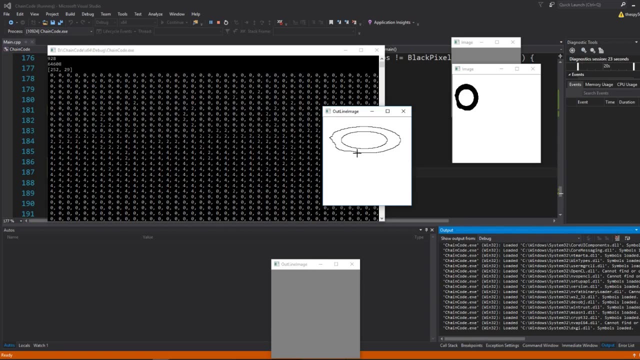 that has the bottoms chopped off this is the outline that the program creates what it says is it starts off down here at the bottom okay we hit zero and we go make this but we start from here and we go down right go across and see the twos get sprinkled around go up up up up up up 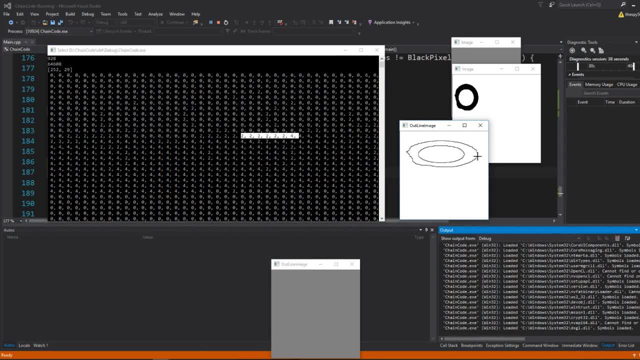 and then eventually we hit a bunch of twos we can assume it's this point right here of the image and then we go west two west two and then we slowly traverse back up 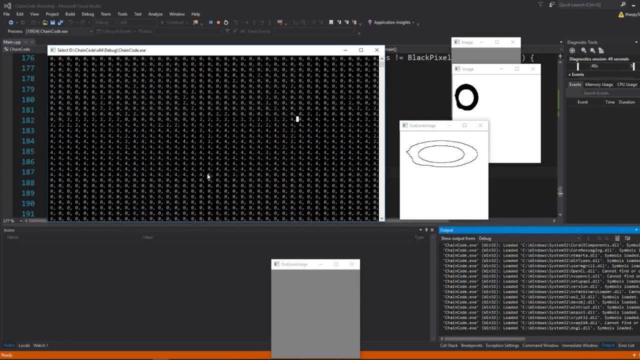 and then we go west and then down with sixes now you see six is sprinkled around